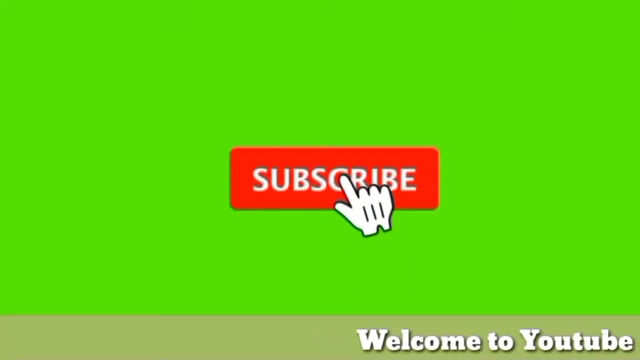 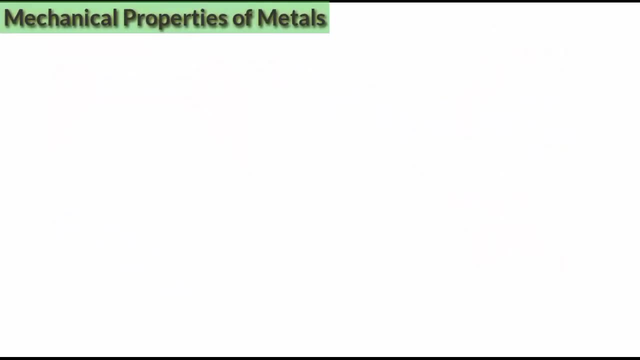 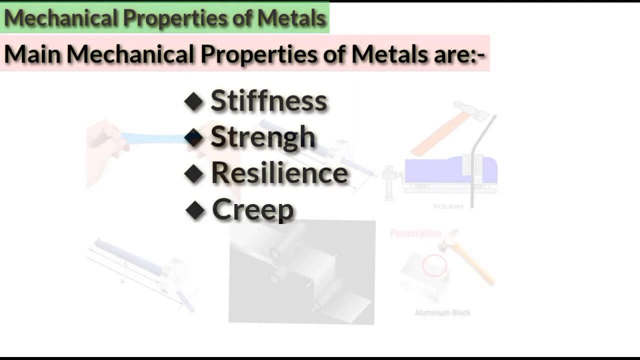 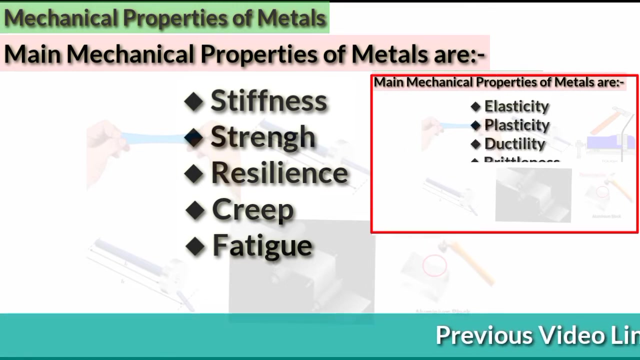 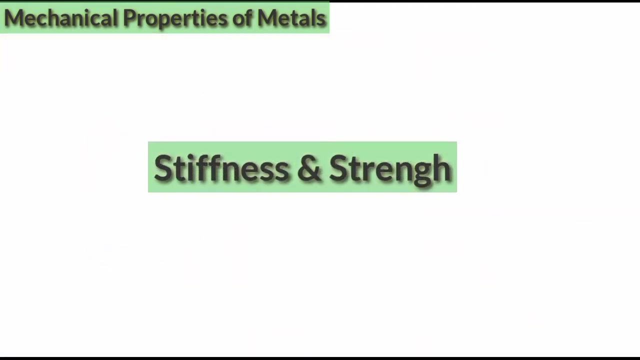 Welcome to my youtube channel, smart engineer. Today we will study about main mechanical property of metal. Some main mechanical property of metal are stiffness, strength, resilience, creep and fatigue. For remaining mechanical property of metal, you can watch my previous video by clicking on i button. First we study about stiffness and strength. 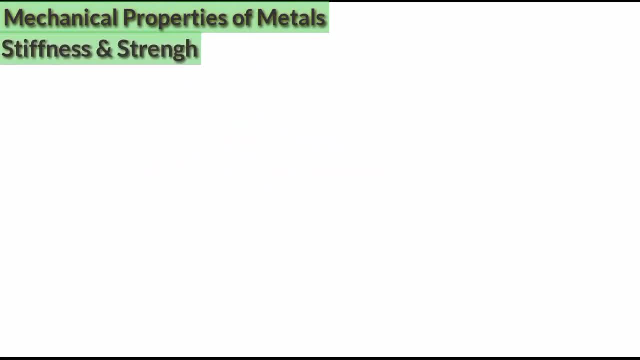 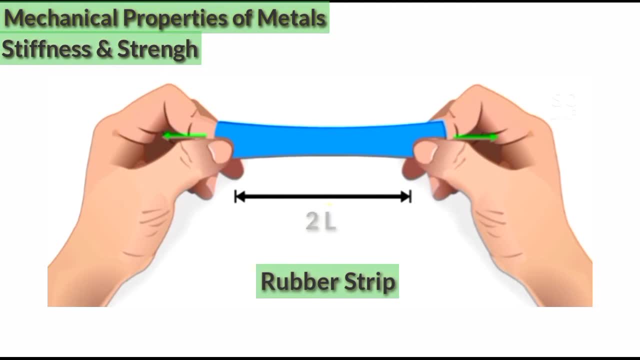 To understand the concept of stiffness and strength, consider a rubber strip. When we start stretching this rubber strip, it can stretch up to a double of its length and then fail. Here we denote the load by A where rubber strip get fail. Similarly, consider a thread. When we start stretching thread, we see thread. 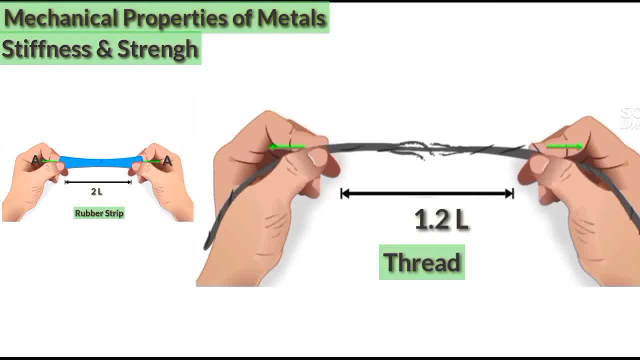 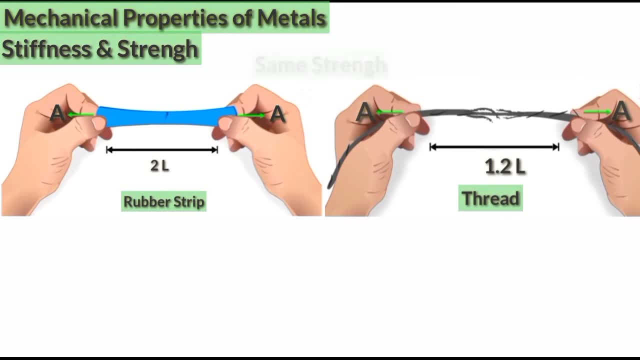 get stretch up to 1.2 of its length and then fillet- same load at A. Here rubber strip and threads get fillet- same load A. Therefore they have same strength. So strength is the ability of material to sustain load without distortion or break. The stronger the material. 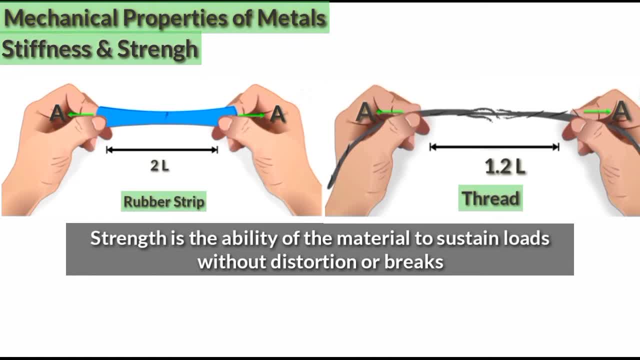 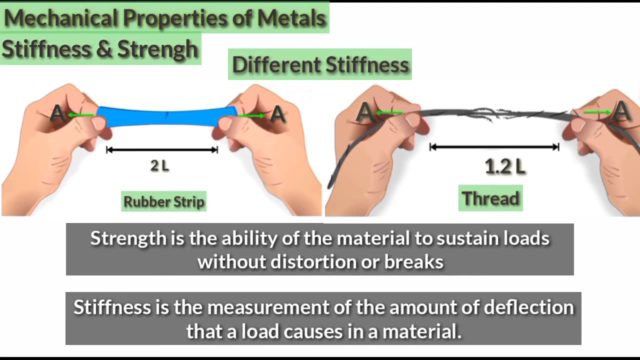 the greater the load it can withstand. Here we also seen that deformation in the length of both rubber strip and the thread is different, So they have different stiffness. So stiffness is defined as the measurement of amount of deflection that a load cause in a material. 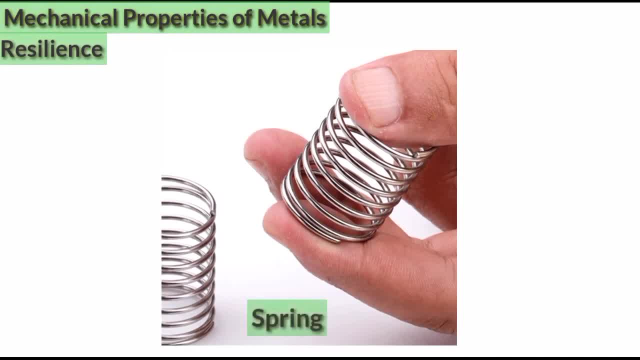 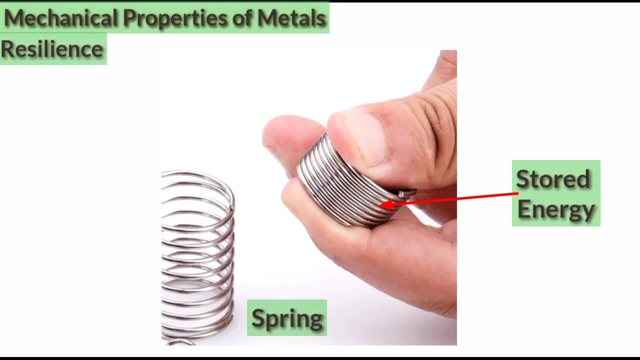 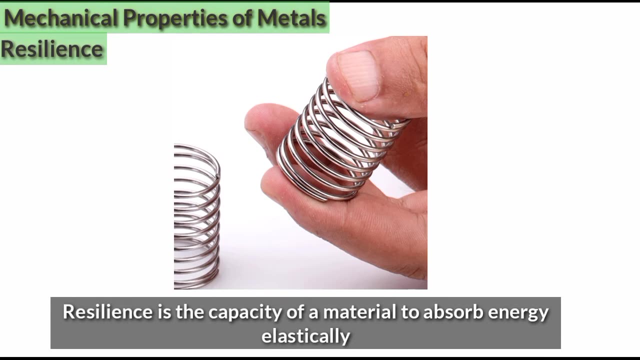 Resilience. To understand resilience, let's take an example of spring. When we apply some load on spring, it's deform and store some energy in it. When we remove this load, spring gets into its original shape. So we can say that resilience is the capacity of material to absorb energy elastically. This property of material is: 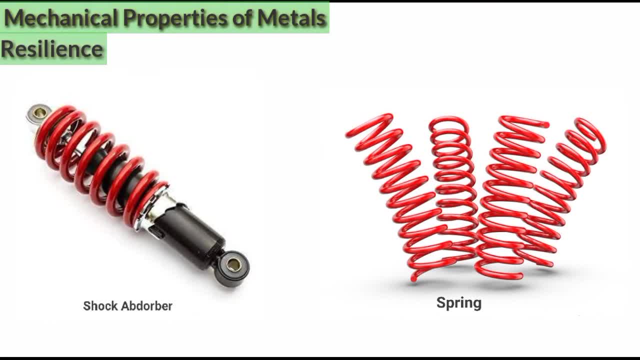 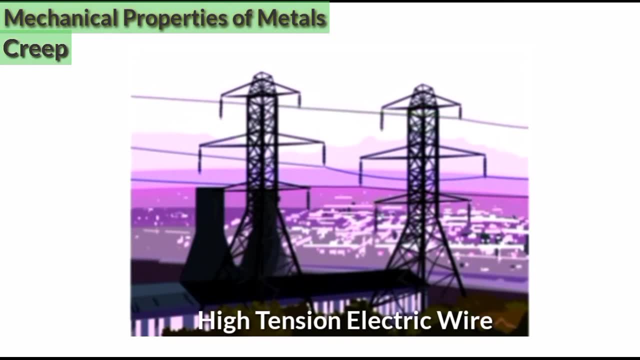 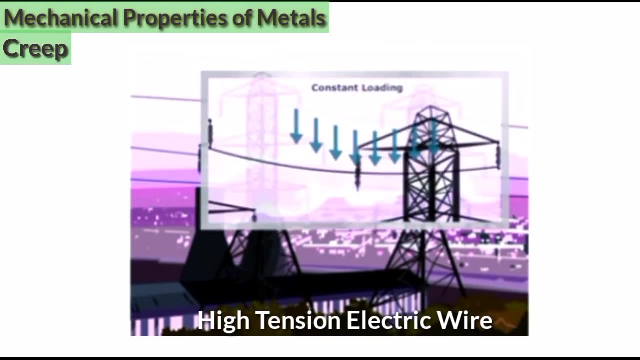 important in the manufacturing of shock absorber and spring Creep. To understand creep, let's take an example of high tension electrical wire. as shown Our span of time, these wires shake due to their constant weight that acts continuously. So we can say that creep is a slow plastic.